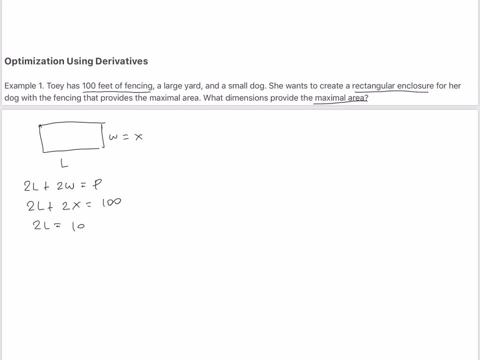 l in terms of x. So we have: 2l is equal to 100 minus 2x. So l is 100 minus 2x divided by 2.. So our length will be 50 minus x. So area of the rectangle is length times width. 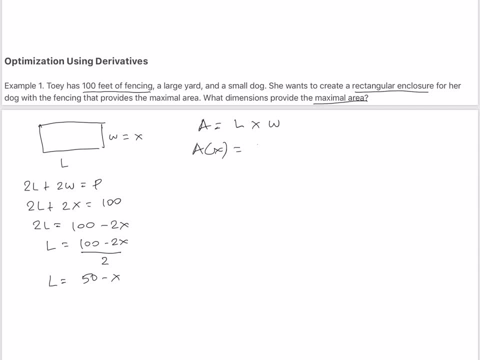 So the area function in terms of x will be 50 minus x multiplied by x. That will give us 50x minus x squared and taking the derivative of that area function, we will have 50 minus 2x And to get the critical value we equate the gradient function into 0 to solve for x. 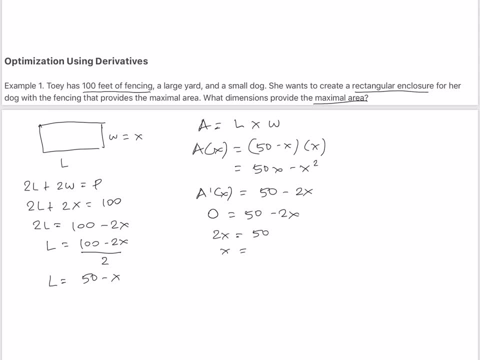 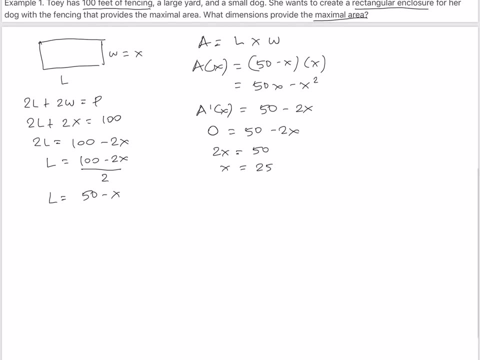 So we have: 2x is equal to 50, x will be equal to 25.. So we got: x is equal to 25, but let us check if that is really a critical value or a maximum. So we have x is equal to 25.. 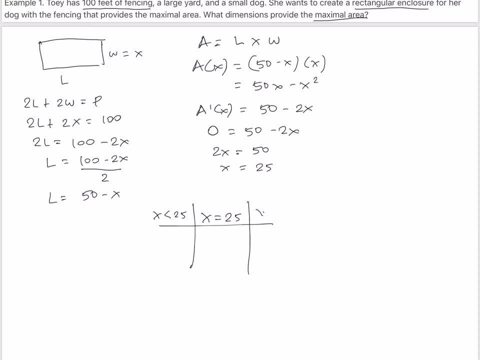 So we have: x is less than 25 on the left and x is more than 25 on the right, So we choose 24 on the left. So we have to substitute. So we substitute that into the gradient function. So we have 50 minus 2 times 24.. 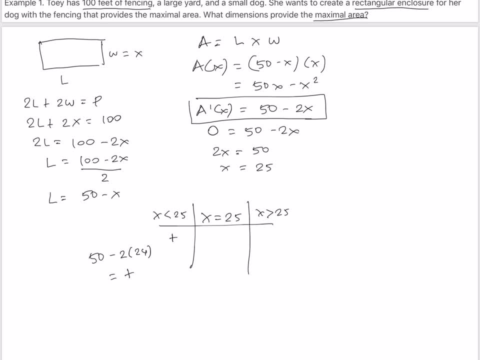 That will give us a positive number here. And when x is 25,, of course our gradient is equal to 0. And x is more than 25, so we choose 26.. So we have 50 minus 2.. Times 26,, that will be a negative number. 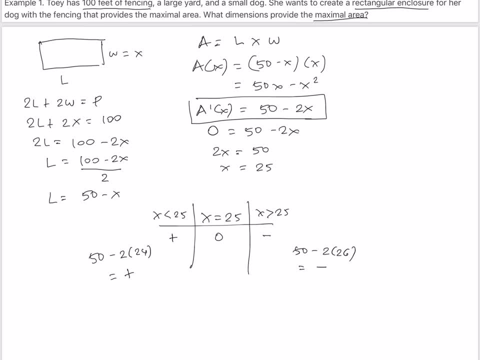 So this one is a negative number. So our gradient here is positive, 0, and negative. So this proves us that 25 is a maximum critical value. So our width now is 25 feet And our length here from 50 minus x.